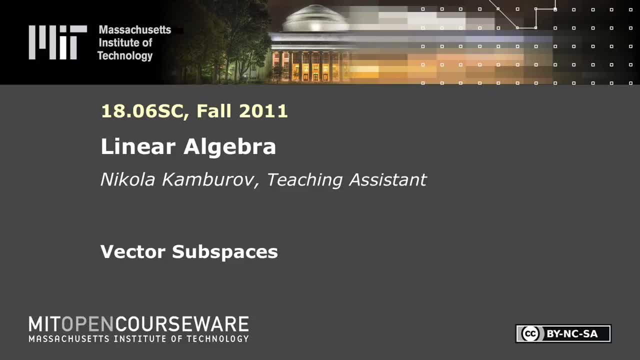 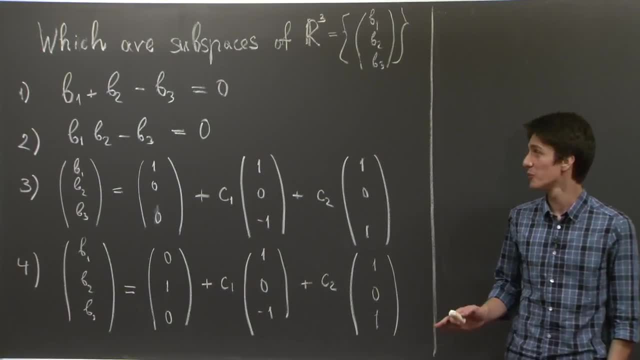 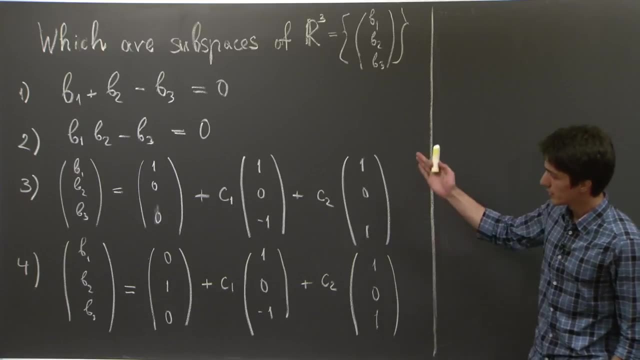 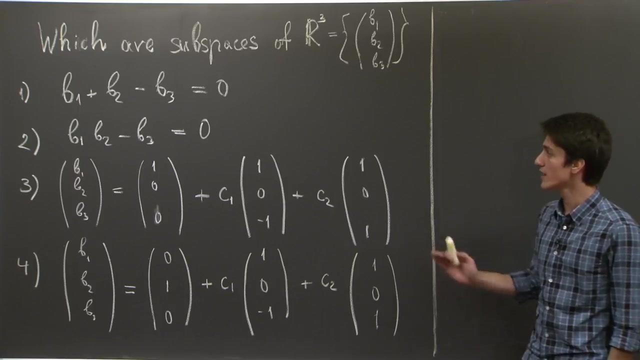 Hi everyone. In this video we're going to explore briefly the concept of a vector subspace. This is the problem that we're going to do. We're given these four different subsets of R3, and we are asked to figure out which of these is in fact a subspace. 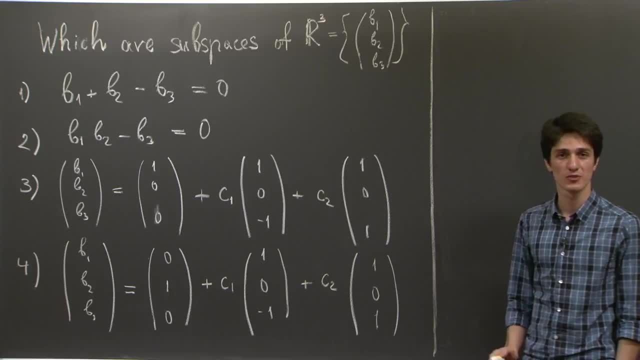 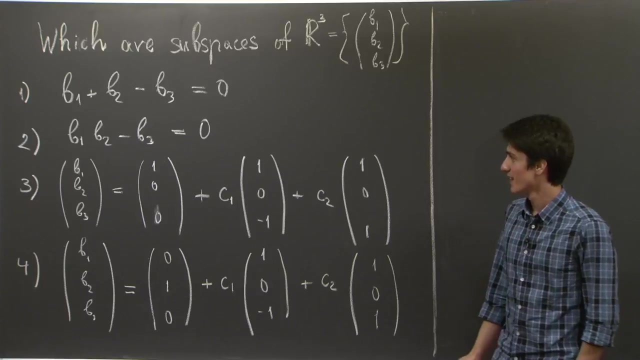 So I'll give you a few moments to try to do this on your own, and then please come back to see whether you are right. So hi again, Okay. so before we start, let's briefly, Let's briefly recall what a vector subspace is. 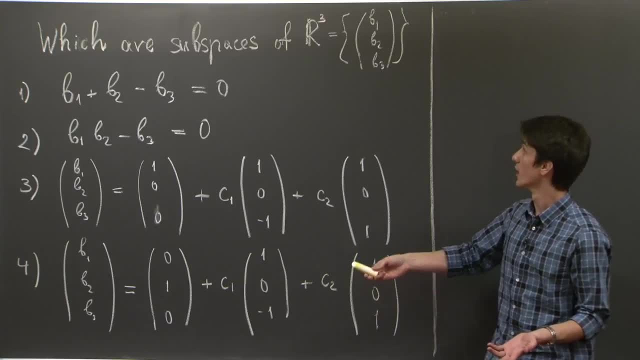 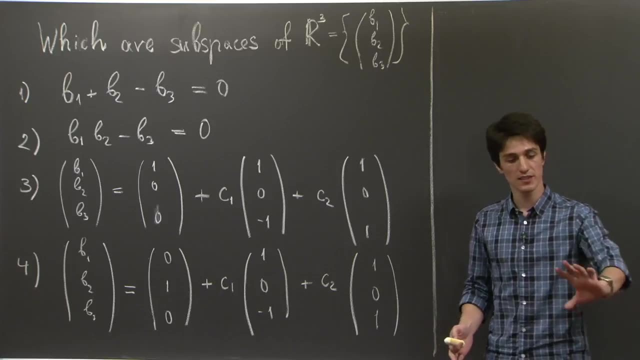 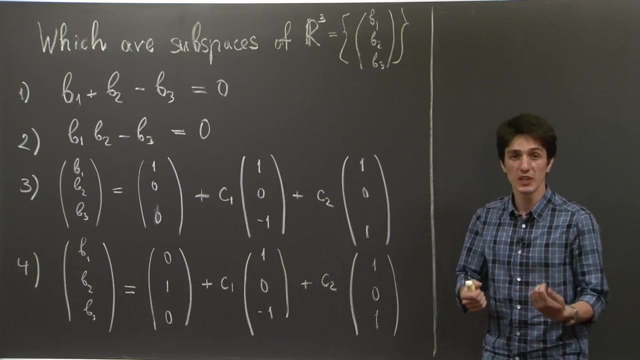 Well, vector subspace. of course it's a subset- in this case a subset of R3, but it behaves like a vector space itself, meaning that if we take a linear combination of elements in this subset, what we get is still something in that subset. 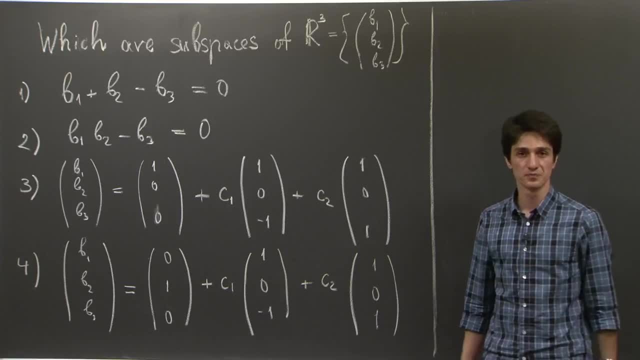 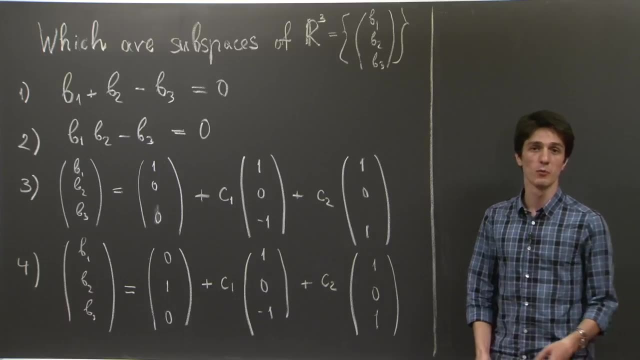 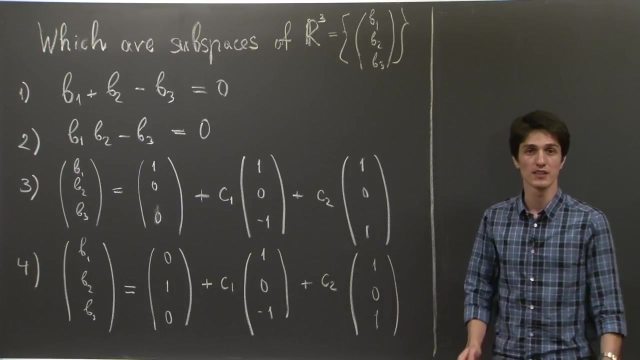 Okay, and in class, Professor Strang showed you a few specific examples of subspaces which are related to matrices. One of them was the null space of a matrix, all the vectors that the matrix sends to zero and the column space of a matrix. 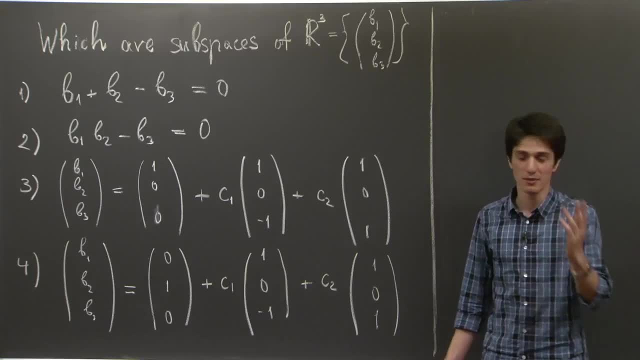 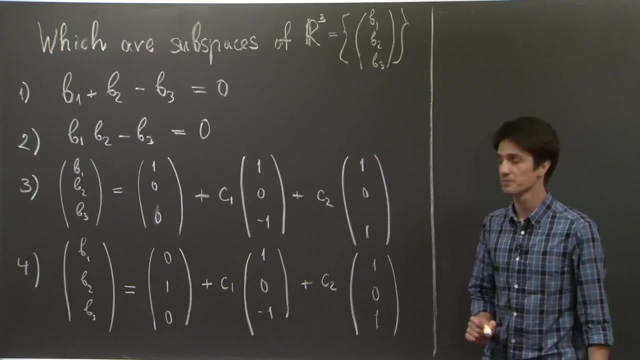 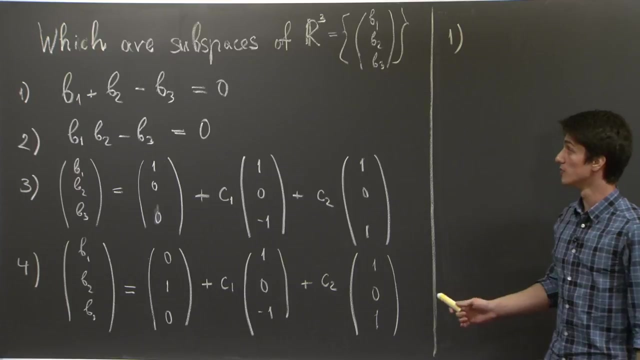 which is the span of the column matrix. Okay, so let's see if we can apply what we've learned in lecture to our problem Number one. we are given a linear equation relation between b1, b2, and b3.. Once we have something linear, we know. this is a philosophy that you'll learn in this class. 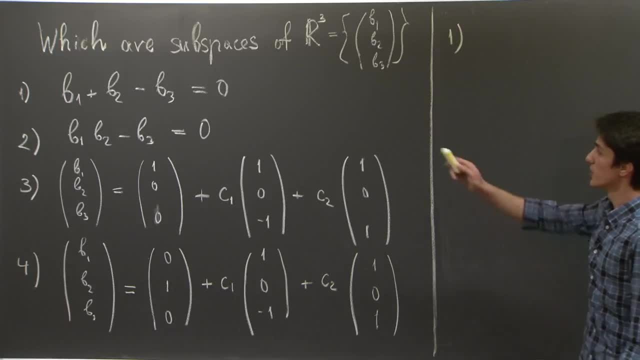 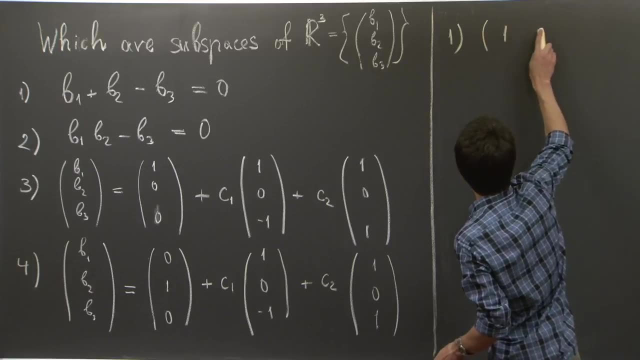 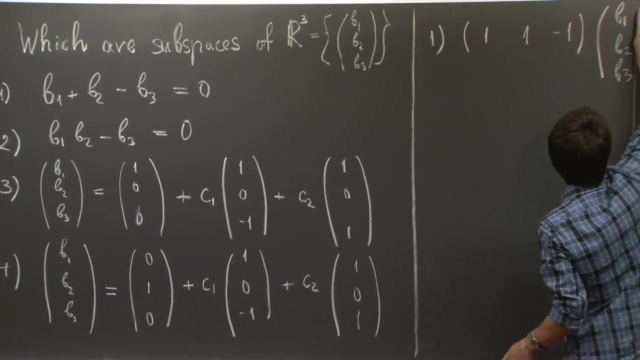 we can always write this as a matrix equation, So in particular, b1 plus b2 minus b3 equals zero. we can just write it as the matrix 1, 1, negative, 1 times b1,, b2, b3 equal to zero. 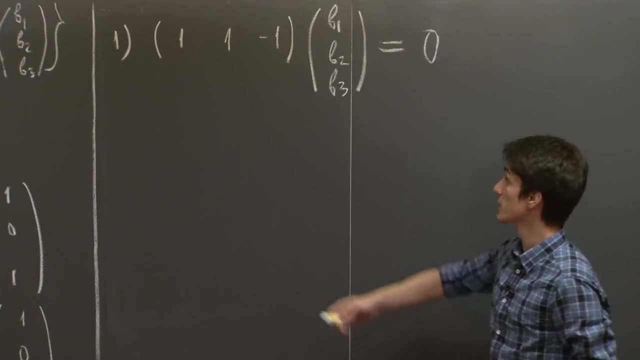 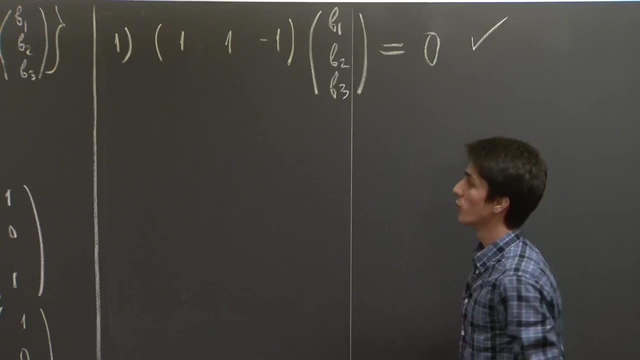 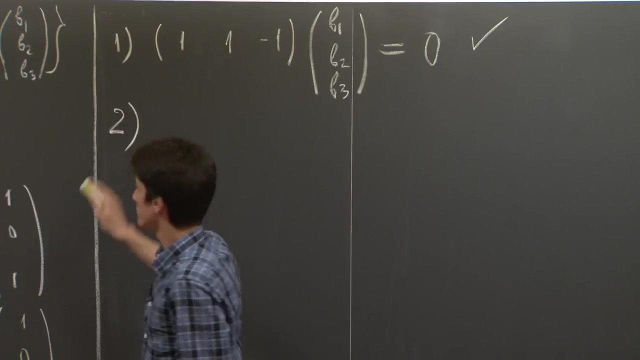 So therefore, b1,, b2, and b3 precisely describe the null space of 1, 1, negative 1, and thus what we are given in the first question is a subspace. What about the second one? Again, we are given a relation between b1, b2, b3, but it's not linear. 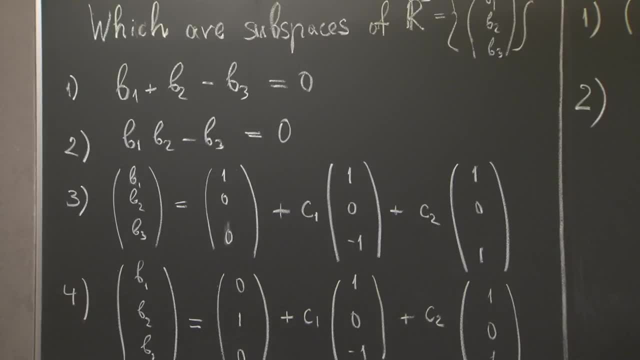 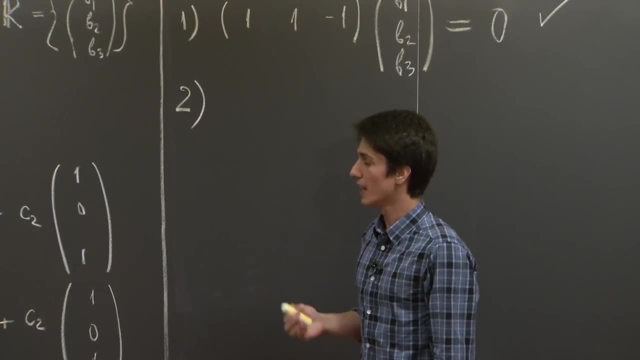 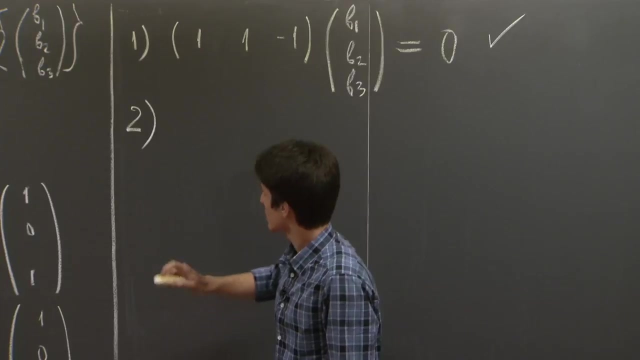 b3 is the product of b1 and b2.. So right, your guts tell you that this shouldn't be a vector space, And we need to, but we need to prove why. Okay, well, see that the vector 1, 1, 1. 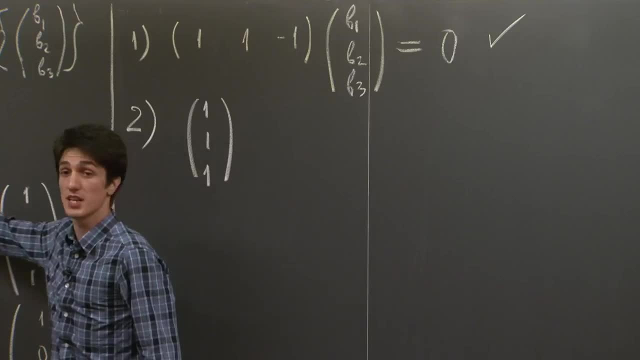 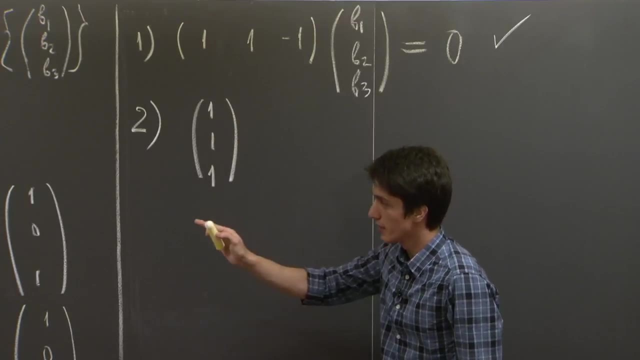 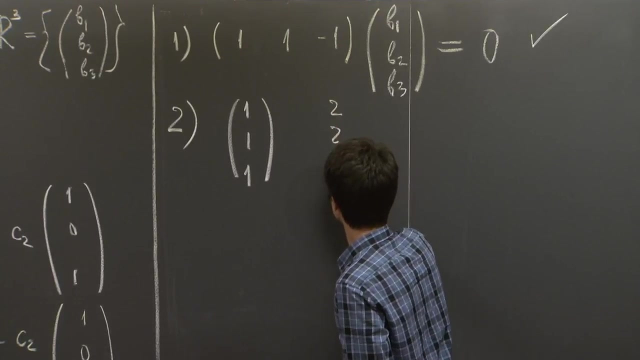 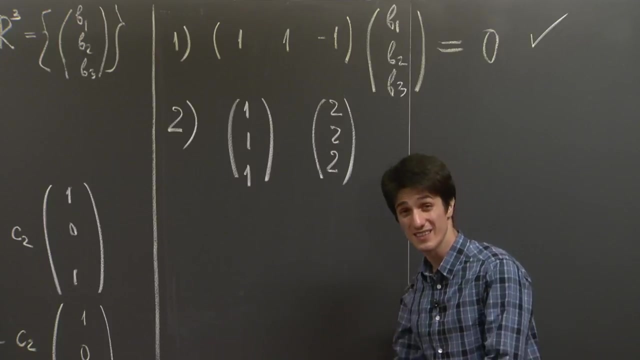 is inside this subset because the third entry is the product 1.. If this subset were a subspace itself, then we would have 2,, 2, and 2 in it as well. Right, Because any multiple of a vector in the subspace is inside the subspace. 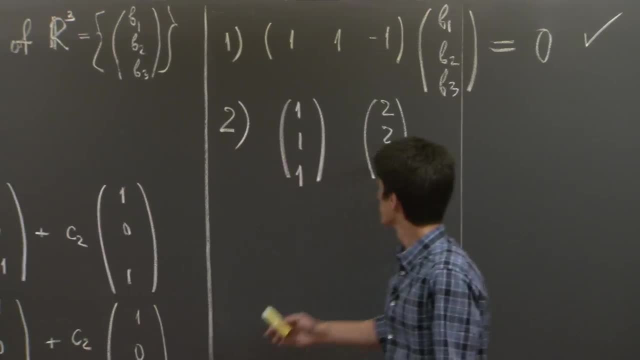 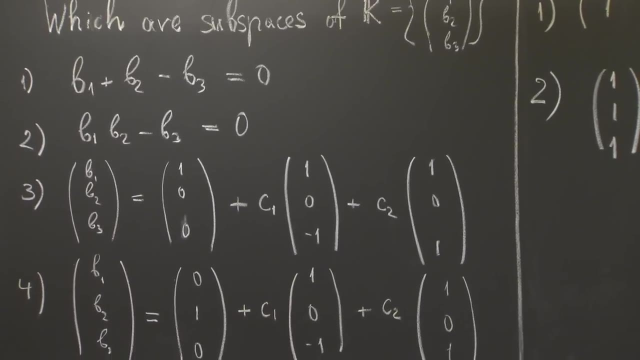 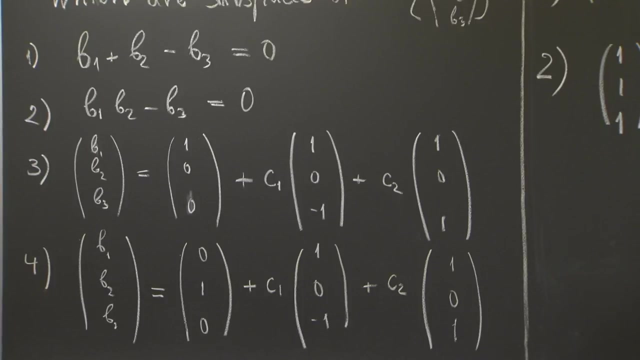 But is 2,, 2, 2 described by this equation? Well, no, because the third entry, 2, is not equal to 2 times 2.. So the example in number 2 is not subspace, OK. 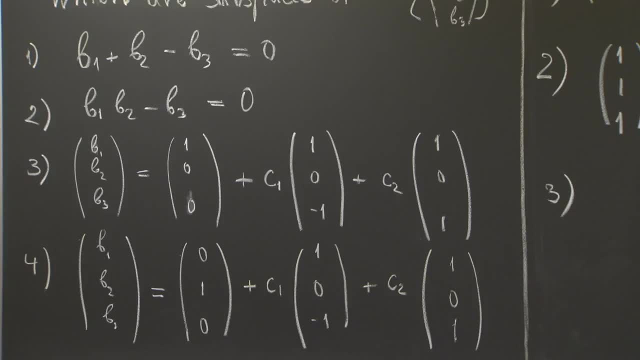 Let's try 3.. And first, so we are given the subset in question. 3 is given as the linear span of these two vectors: 1, 0, negative 1, and 1, 0, 1, plus the vector 1, 0, 0.. 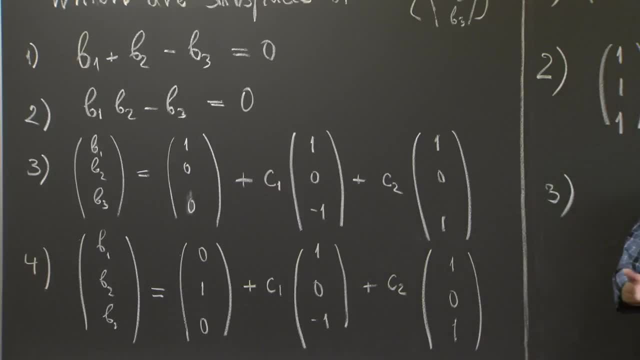 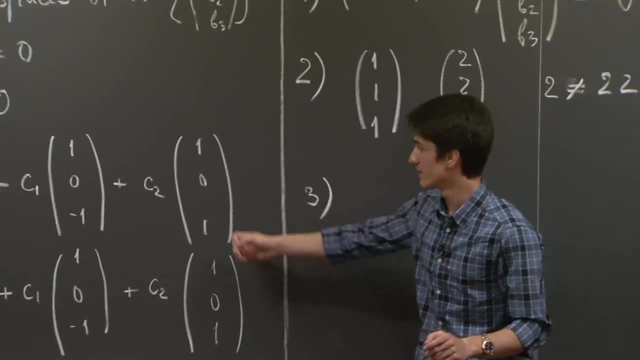 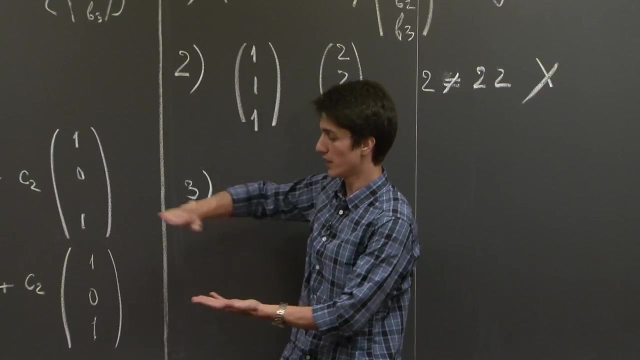 OK, So let's think about this geometrically. We know that the linear span of two linearly independent vectors, And- And these are obviously linearly independent- is a plane in R3.. So we have the plane And we add a vector to the points on this plane. 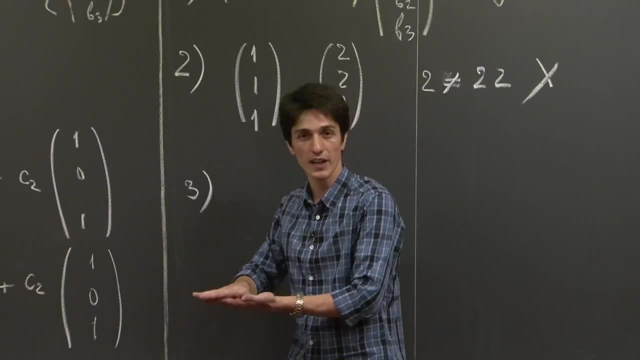 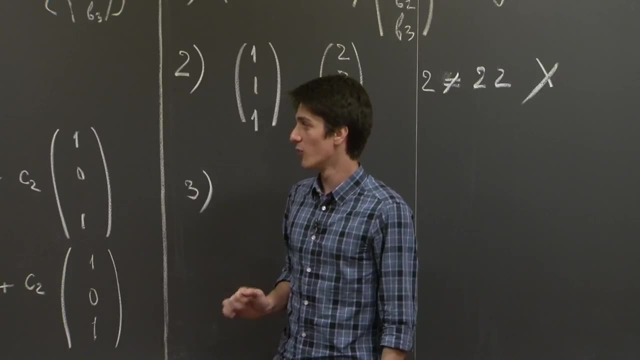 So what if the vector were lying on the plane? Well, we're not going to change the plane right? We're still going to remain in the plane. What I'm hinting at is the following thing: that, in fact, 1, 0, 0.. 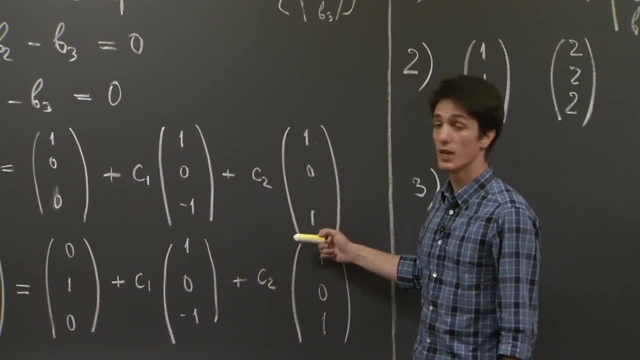 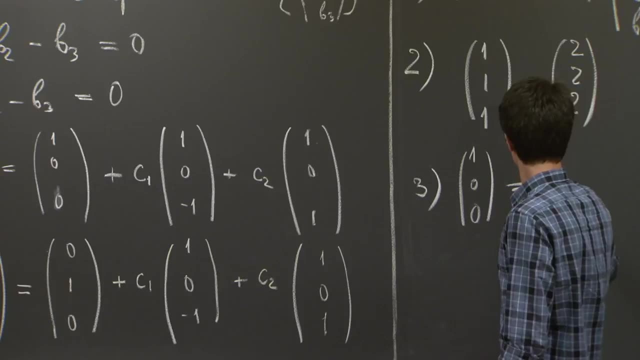 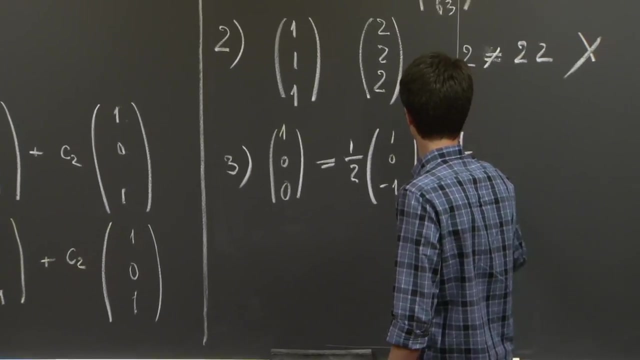 It is a linear combination of 1, 0, negative 1, and 1, 0, 1.. And it's fairly obvious to see which linear combination of these two vectors it is: It's 1, half 1, 0, negative 1, plus 1, half 1, 0, 1.. 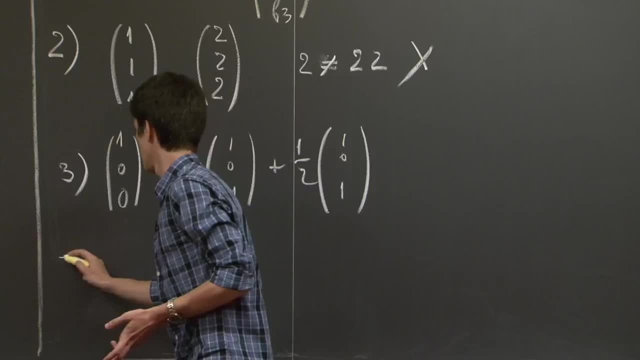 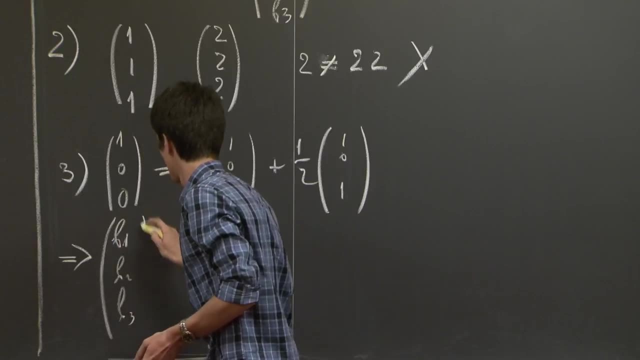 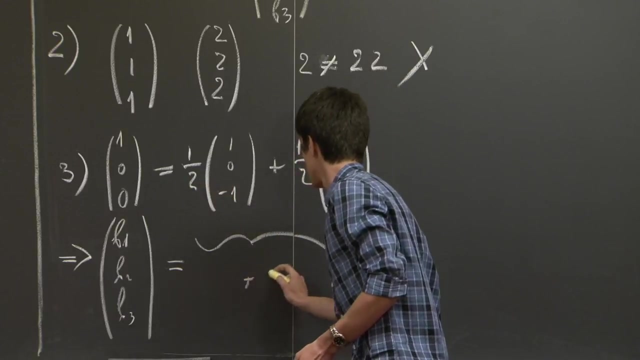 So we can write the whole relation here in the following way: b 1. b 2. b 3. Is 1, 0, 0,, which we can write as this: plus 1, 1, 0, 1,. 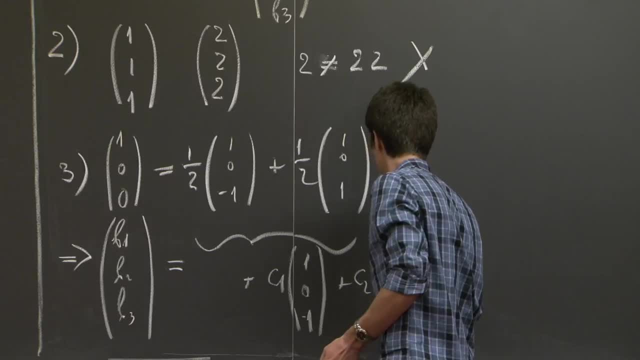 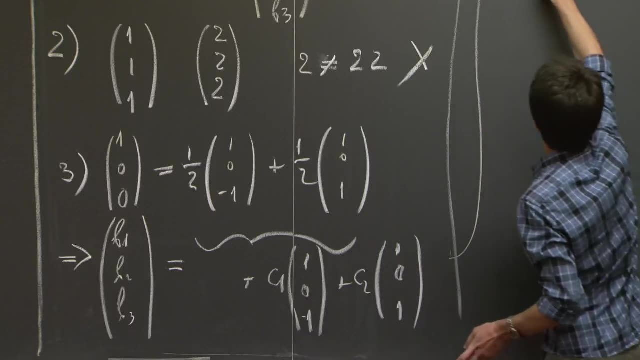 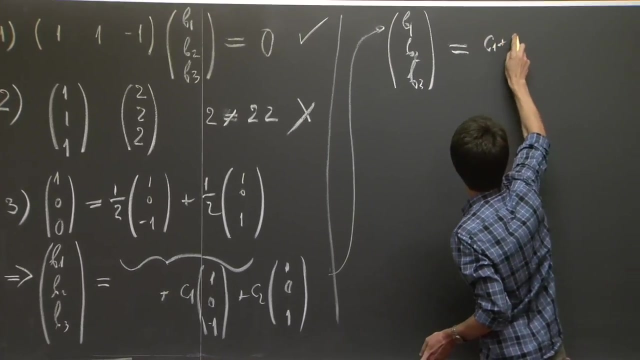 negative 1, and c 2, 1, 0, 1.. And let me continue this here. So b 1,, b 2, and b 3. Is precisely c 1, plus 1, half of 1, 0, 1.. 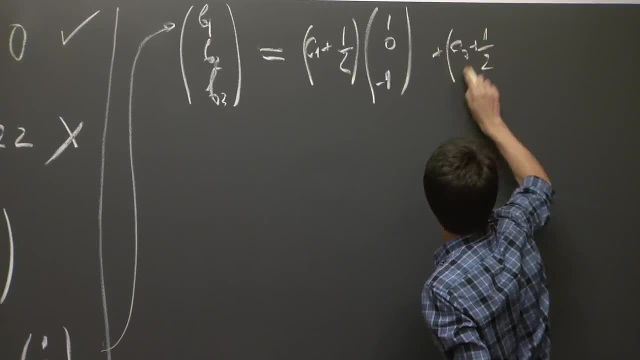 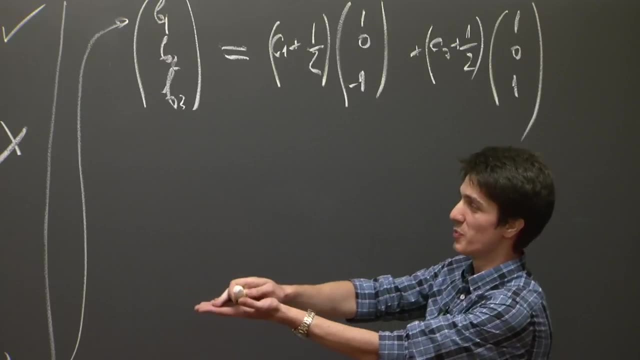 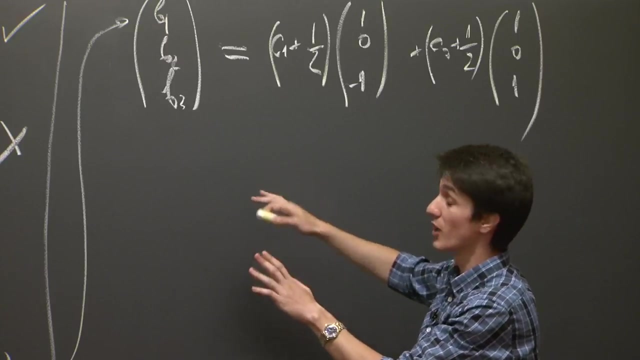 Negative 1 plus c, 2 plus 1, half of 1, 0, 1.. So, indeed, the points b 1,, b 2, and b 3 are described by the linear span of 1, 0, negative 1, and 1, 0,. 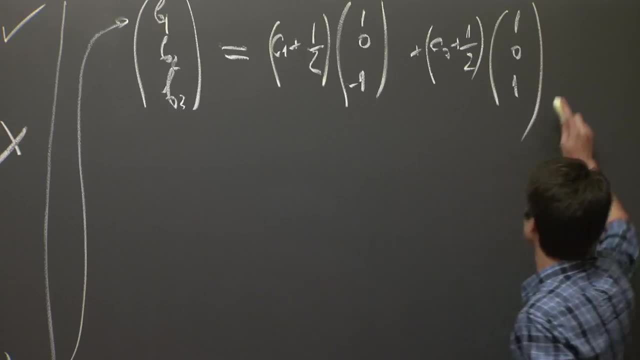 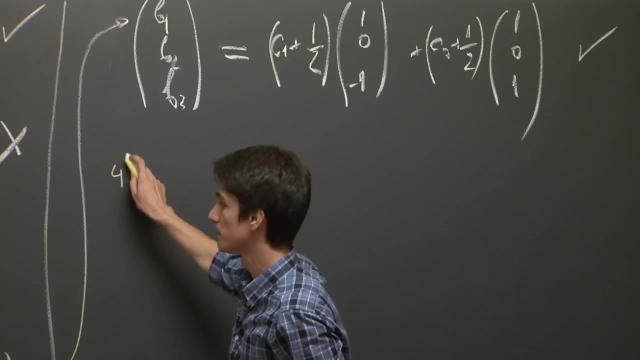 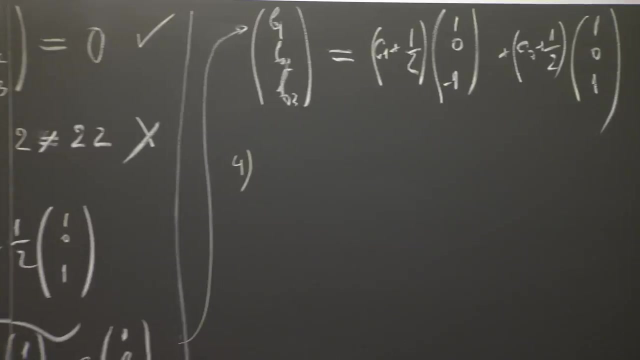 1. So it is a vector subspace itself. And finally, let's look at number four. So we have a similar situation. I mean it's almost the same situation. We again have the linear span of precisely the same vectors as in question three. 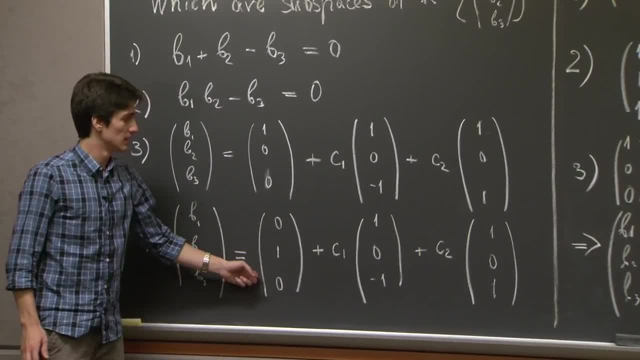 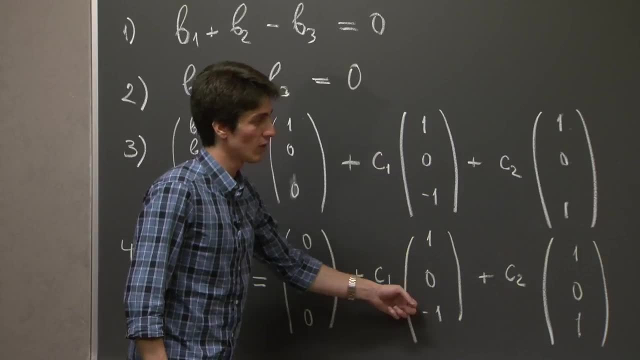 But this time we add the vector 0, 1, 0 to them. Now 0, 1, 0 is not 0.0.. 0, 1, 0. in the span of these two vectors. So the argument that we just showed for 3.